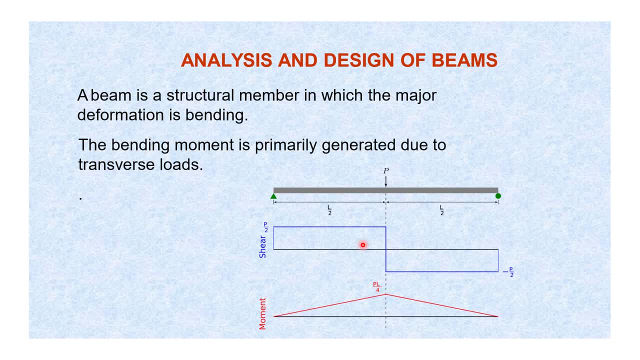 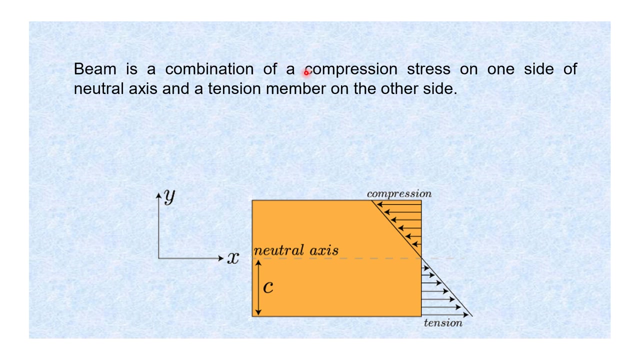 moment. then we will check for shear force and we have heard we have to also satisfy the shear criteria. the bending moment is primarily generated due to the transfer load that is acting up downward on the beam beam. when I loading act on a beam, then a combination of stresses form that above the neutral axis compression. 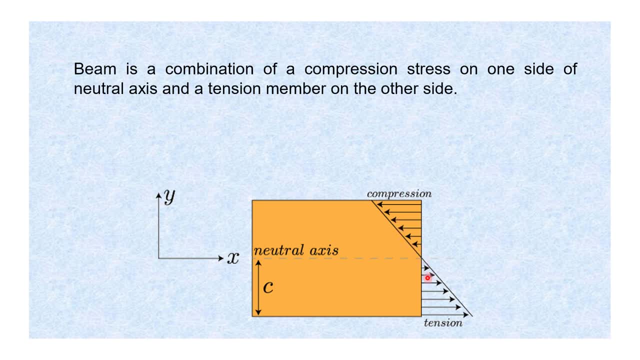 stress will generate and below the neutral axis, tension stress will generate. and one thing more: in steel members that are strong in compression as well as in tension. so there is a no issue of steel is weak in tension. steel is strong is in compression and steel is also strong in tension. here is a 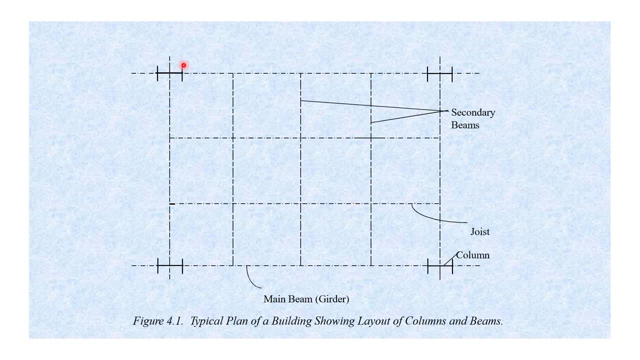 overview of the plan of steel building. okay, here you are seeing four columns. okay, I shape column and the columns which are connecting with the lines, these are beams. okay, the these are main beams that are running above the columns. so these are main beams and the main beams beams. 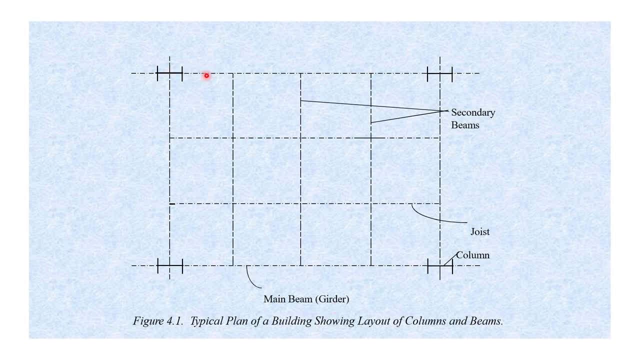 are also called girders, and the beams which are connecting the main beam to the other main beam that are secondary beam. this is secondary beam but the hair is small that is connecting main beam to this can be beam that is joist, that is, less important beams. but with the help of 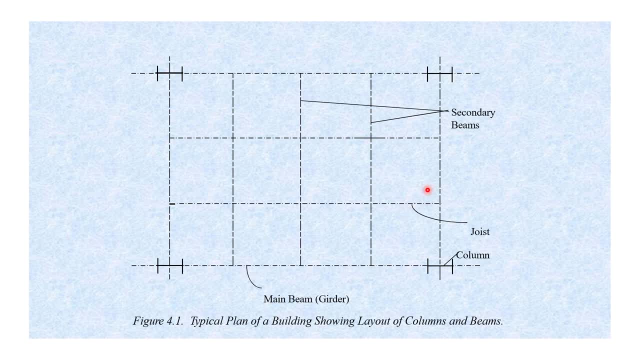 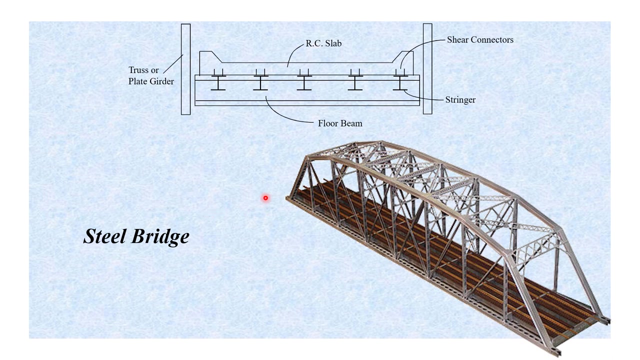 that we get the favor in the designing of slabs in. then the shears, the strength, the deformation and all things will be improved due to this beam beam phenomena and we need less depth of slab due to this beam arrangement. here is a steel bridge. okay, here is a rust steel bridge and here is a cross section. before going, 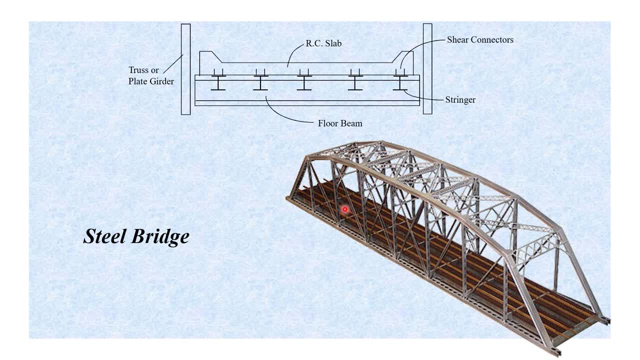 to the cross section. first, see, here you are saying that there are longitudinal beams and here horizontal beams. okay, and all these longitudinal beams are resting on this horizontal beam. same, these longitudinal beam that are resting on this horizontal beam, that is horizontal beam, that is called floor beam, and these 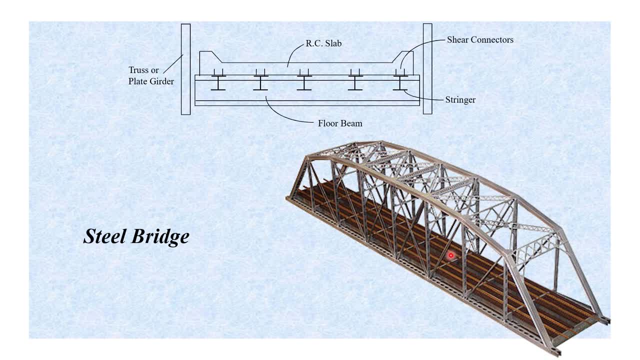 longitudinal beams that are called stringers and after this longitudinal beam Resting on the floor beam, then the ultimately floor beam are resting on this truss joints and from The loading from this truss joints will transfer ultimately to the sports. So that is the phenomena of load transfer in the truss bridge. 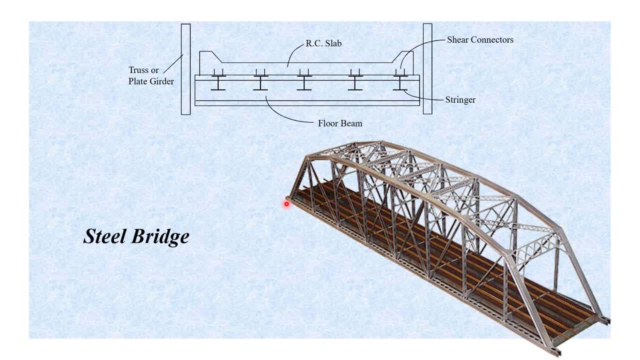 in case of steel bridge and On this side there is maybe a truss or there may be large size steel girder or steel beam. So here on the left or right side there may be truss or plate girder. That is a heavy player girder is a heavy beam. 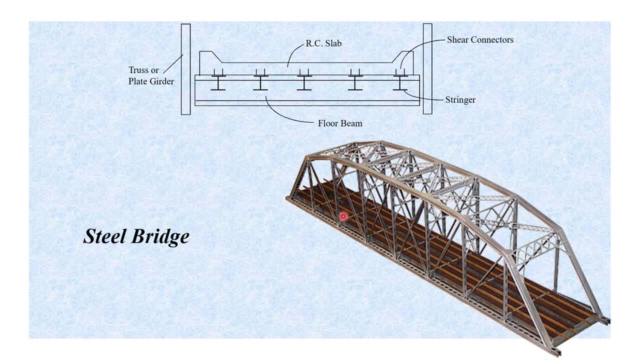 that is a built-up section and Here you are seeing the horizontal Beam. that is a floor beam and on the floor beam there is a stringer. okay, the stringer are resting on the floor beam and this slab is resting on the Stringers. and stringers are connecting to the slab with the shear keys and shear starts. 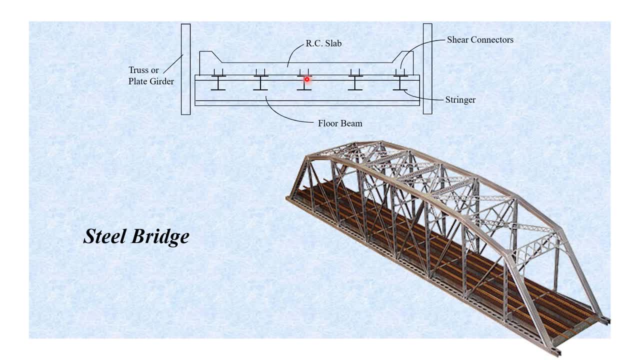 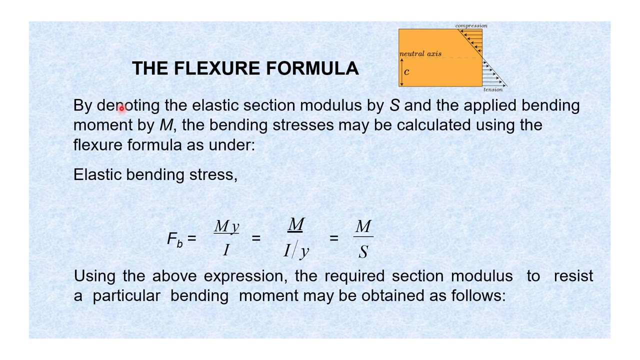 That are just like balls are welded on the steel beams and so that the good connection dwell between the concrete and steel. The flex, your formula, the basic formula for the beam, for the flow, your stresses, by denoting the elastic section, modulus s and the applied bending moment, by 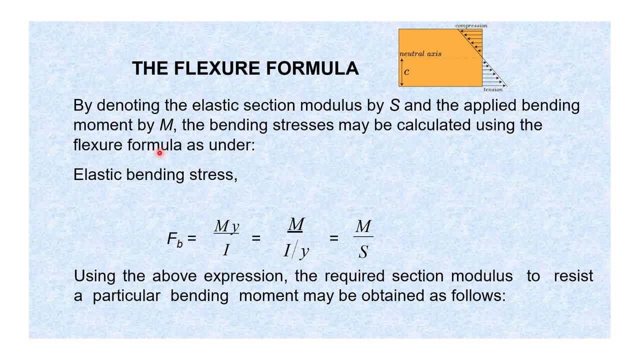 M. the bending stresses may be calculated using the flex, your formula, as under elastic bending stress basic formula. that is basic bending stresses in beam, that is, movement y over I. why is the distance from the center, from the neutral axis, to the Up Toe fiber or wherever you want to find this stress? 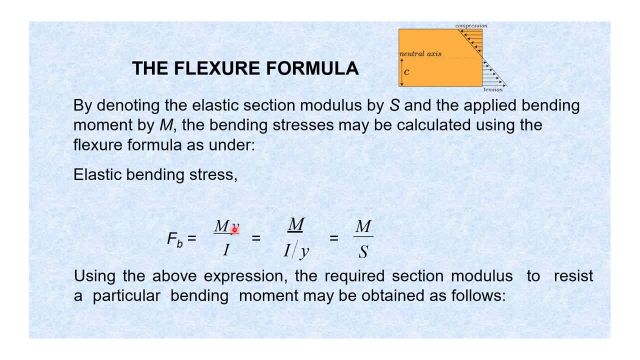 Okay, here that is a, C and in the formula that is y. so that is the same. I is the moment of inertia. if we divide I by Y, then I or Y is the. Is this section modulus? and using the above formula, The required section modulus to resist a particular bending moment may be obtained as follows. for example, from the analysis of beam, 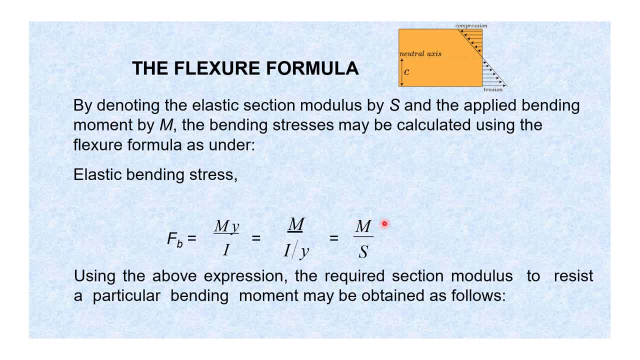 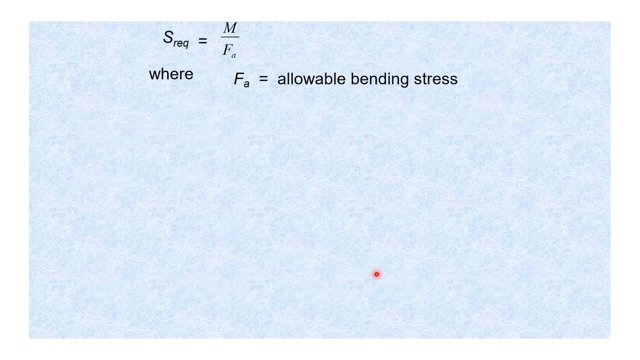 You got the applied moment but and you also know the beam Allowable stress, then you, if you know the moment, the allowable stress, Then you can calculate the required section modulus. you can take s on the other side and F to the bottom, M over F. Here again, s required equal to M over F a, where F a is the allowable bending stress. 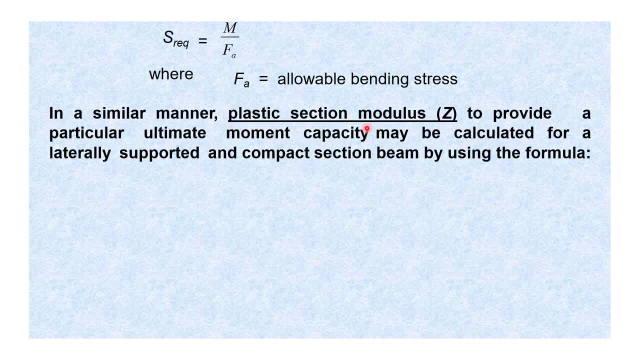 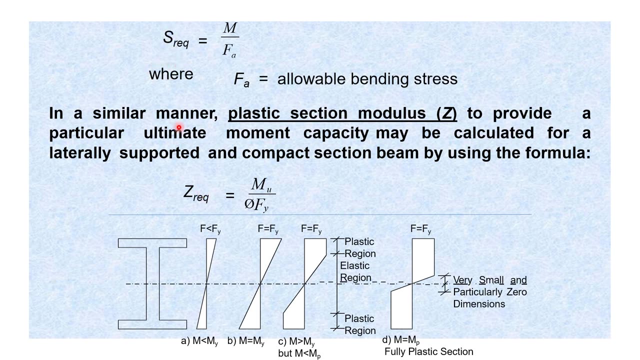 in a similar member a manner. plastic section modulus to provide a particular ultimate Moment capacity may be calculated for a laterally supported and compact section by using the formula this: Here is the elastic section modulus s. there is a plastic section modulus that we can calculate from again same formula applied moment. here is the yield strength and 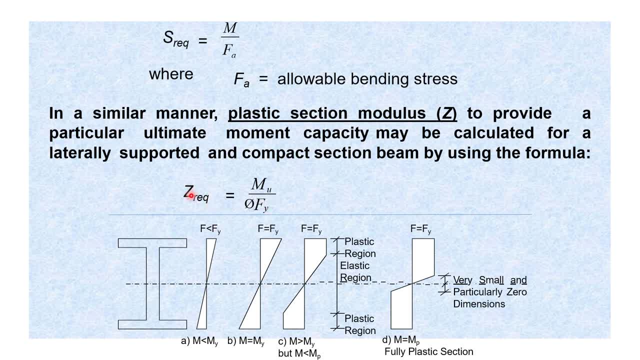 What is the plastic section modulus there? Here you can see the stress profile, stress applied in a beam, and if that is Less than yield stress, this diagram will become. when the stress equal to yield, then this diagram will become when the yielding start. then first extreme fiber start yielding, then other. 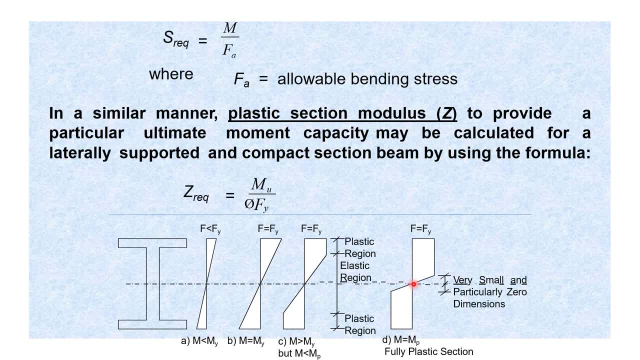 bottom fiber yield that ultimately it comes to the Neutral axis, then at that point whole section will Plastify. then at this point this beam will or section will act as a hinge. when we got the section modulus at the elastic range means when in the, When the elastic profile, then that is elastic section modulus and when the section fully plastified. 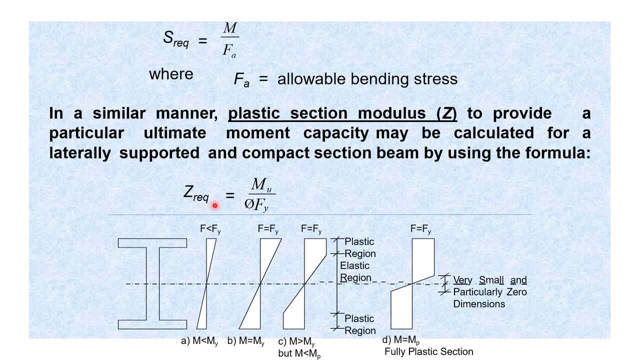 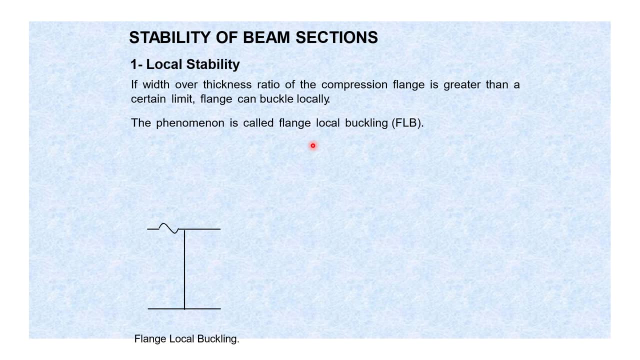 Then at that point, when we calculate the section modulus, at that point the section modulus is plastic section modulus Mean fully plastic section. Stability of beam section. there are different types of stability. I will discuss one by one. first one is the local stability. If the width our thickness ratio, 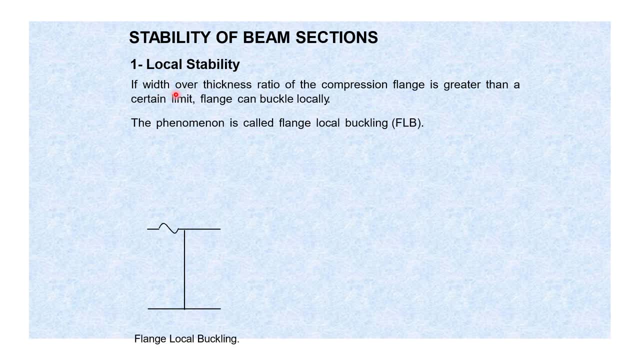 It is just like a slenderness ratio. if the width, our thickness ratio here is the width of this plane, total width of the flank Divided by two, you will get half flange width. half flange width, That is just like a unsported length. and 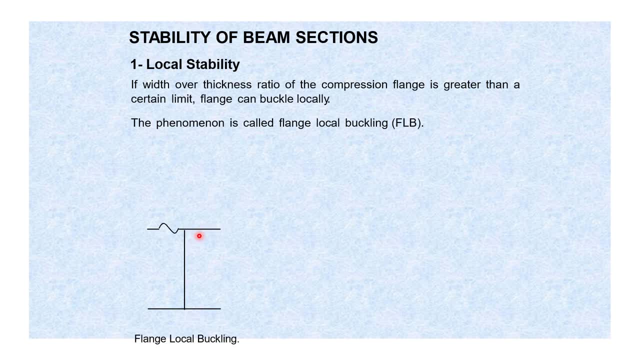 You take the length from this part to this part and divided by thickness, then you will get the slenderness ratio or the ratio value. if, if the width- our thickness ratio- of the compression flange Is greater than a certain limit, flange can buckle locally. means this member can buckle locally, not overall. 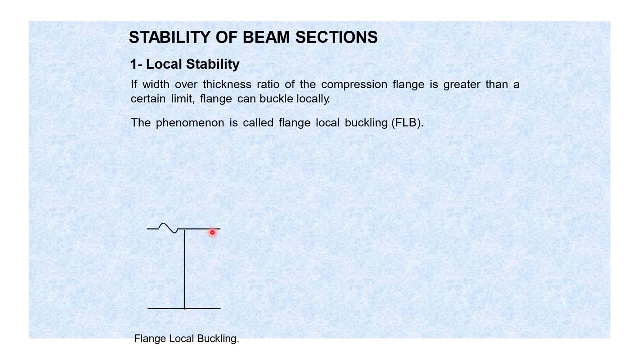 its local size Can triple. can damage by due to the this criteria. If phenomena is called fly local buckling, if there is a chances of buckling in the flange due to certain limit that I will discuss In the next slides. What is the criteria? 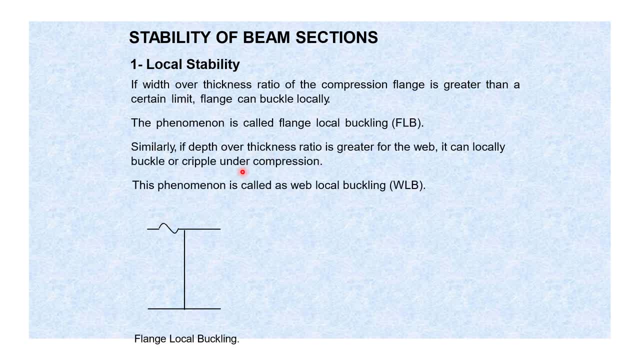 so. so that is flange local buckling. similarly, if depth over thickness ratio is greater for the web, it can buckle or triple under compression, like this: okay, i section and the, the web of the i section may go buckle, so that is called web local buckling. that is web of beam, so that is web local. 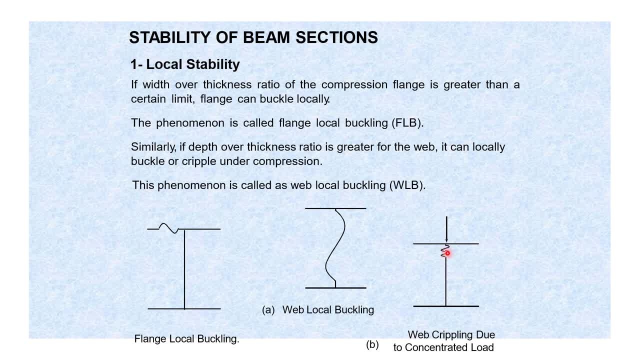 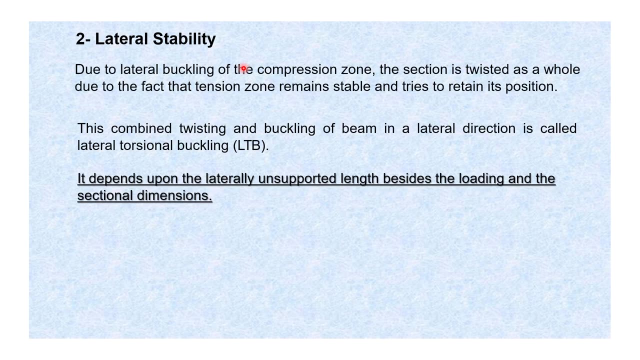 buckling and there is also due to the concentrated load. there may be chance of concentration of large locally damaged. so that is called web crippling due to concentrated load. so that is local stability. so we have to also perform the checks. second one is the lateral stability. due to lateral buckling of compression zone, this section is twisted as a whole due to. 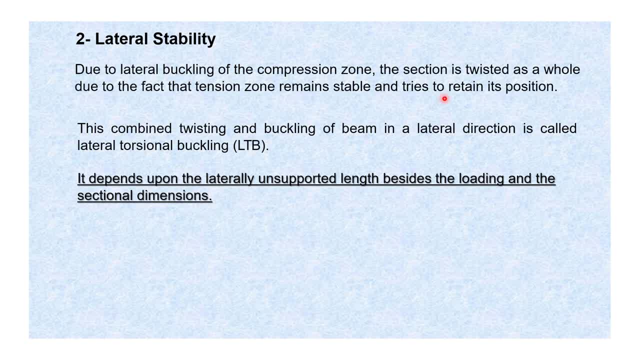 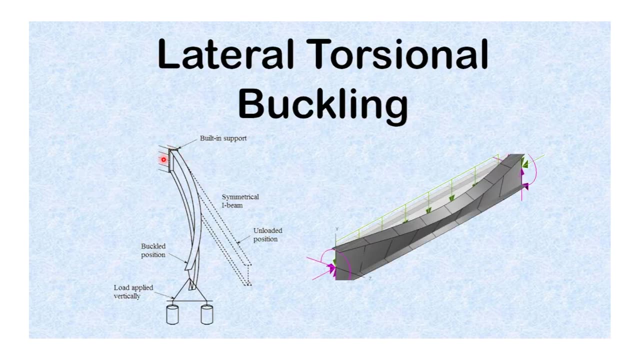 the fact that the tension zone remains stable and tries to retain its position. the combined twisting- okay so- and buckling of a beam, the whole beam in a lateral direction, is called lateral torsional buckling. here here is a beam fixed at one, the other side, one side, and you can say: hinge on the. 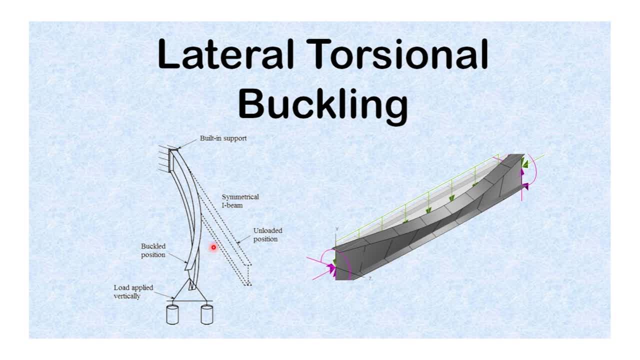 others, uh, on another side, then due to the twisting of this beam- this is called lateral torsional buckling. the member can twist. here is a channel section. when the load applied, the channel has the tendency to twist. so this similarly, i section if the sites where loading is, uh, there is, or there is a eccentricity, anything. 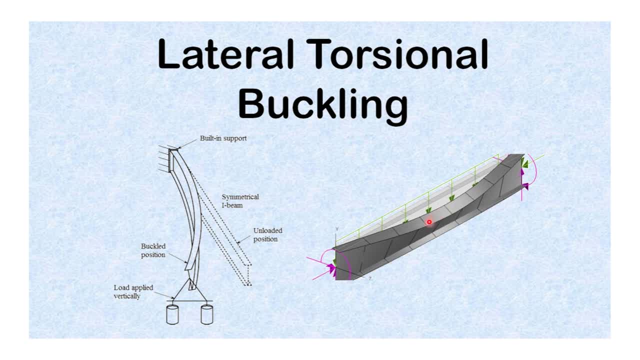 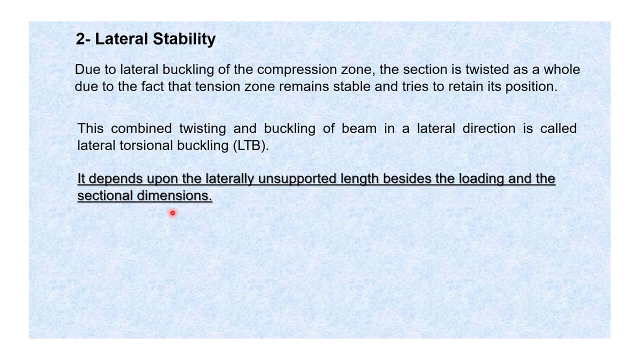 or the charge. there is a lot, much chances that the the beam buckle and twist okay at the same time. this is called lateral torsional buckling. it depends upon the laterally unsported land besides the loading and dimensions and sectional dimensional means. if that is very long beam, then 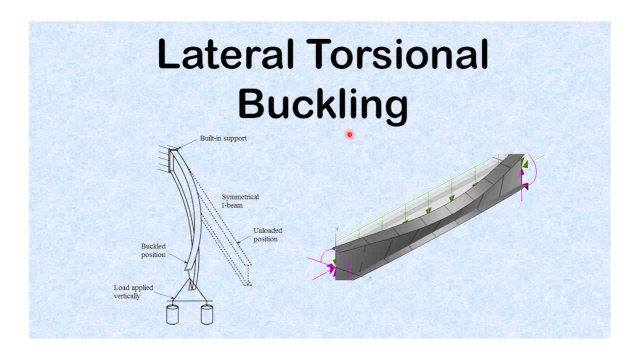 is a much chances that it goes. lateral torsion buckling means their unsupported length matters a lot, okay. so if there is uh, some bracing or some uh arrangement that that can stop the twisting, so that is a uh will be act as a controlling uh, controlling criteria for uh resisting lateral. 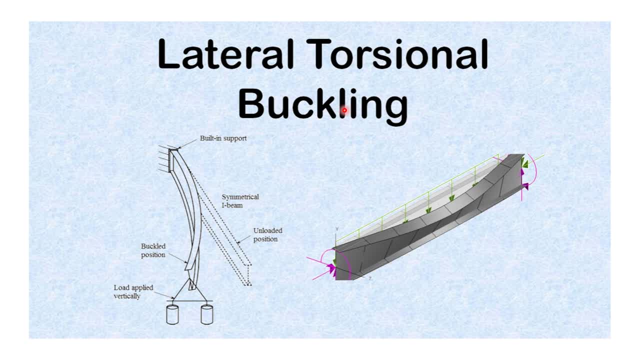 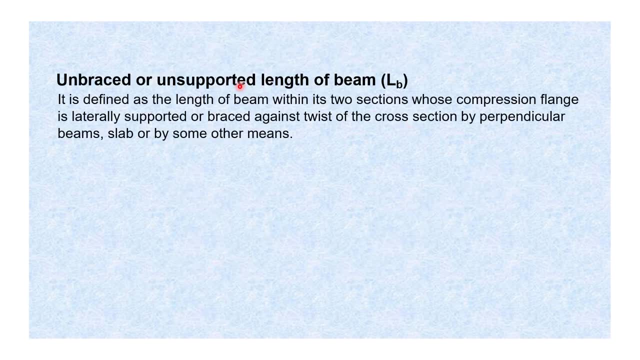 torsion buckling. so again, we will discuss in further uh in and in more detail in the next slides about lateral torsional buckling, unbraced on or unsported length of beam. it is defined as the length of beam within its two sections whose compression flange is laterally supported or 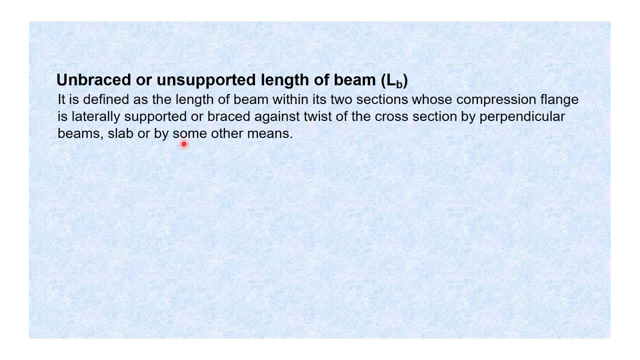 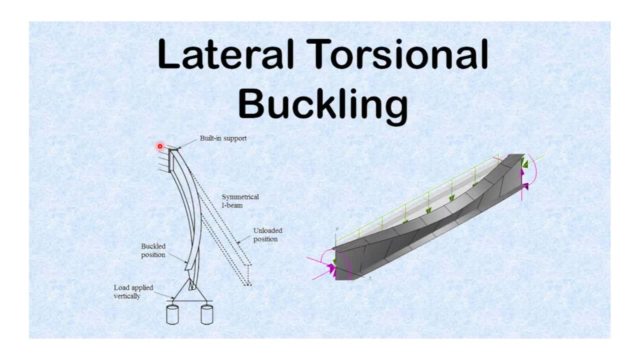 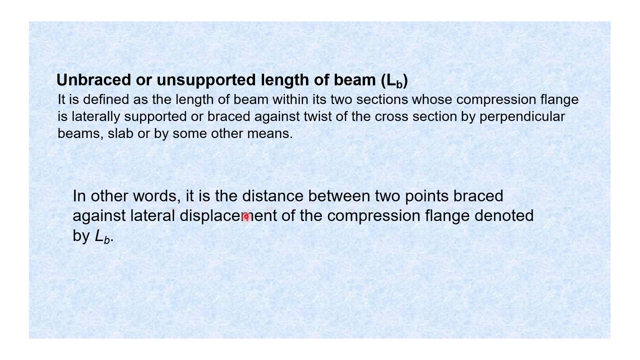 braced against, twist of this cross section by perpendicular beams, slab or by other means. for example, here the unsupported length, here is the sport and here is sport. here is the unsported line in between between two sports. that is a unsported line, if okay, let's see another. in other words, it is the distance between two points based. 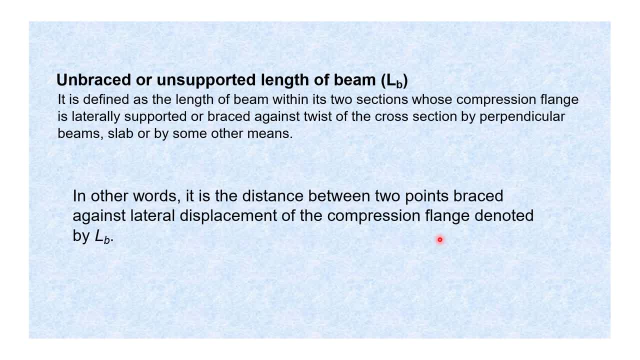 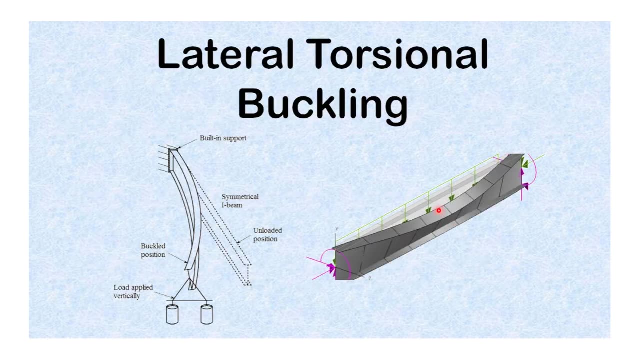 against and lateral displacement of the compression flange denoted by LB. the section brace to prevent twist of the member are considered better for the bracing against the lateral torsional buckling. so if we provide, provide some section here that can resist the twisting due to this lateral member from. 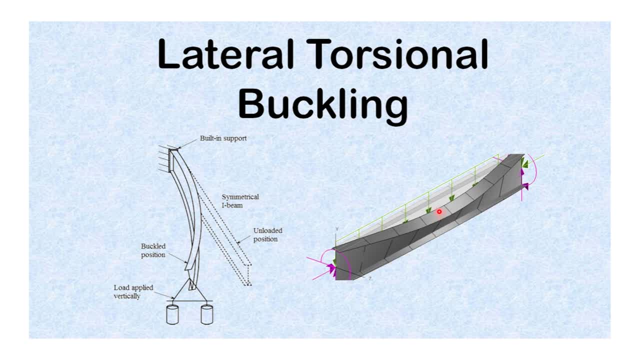 this side or at midpoint, or some bracing, then you can understand, there is a less chances of buckling. so if we go for less unbraced lens, that is good for us. so lateral torsional buckling means that we have to utilize the stripe of the MRB. left brace. but notice that if we remove from thisoke the republic we complicated Keep touching the dog's head. so it's in a second tuning. artists on this side asked that can resist the twisting between along side. therefore, luckily, if under steps, maybe unt Circo Lesmond and cross the left arm and bring down a here receiving. 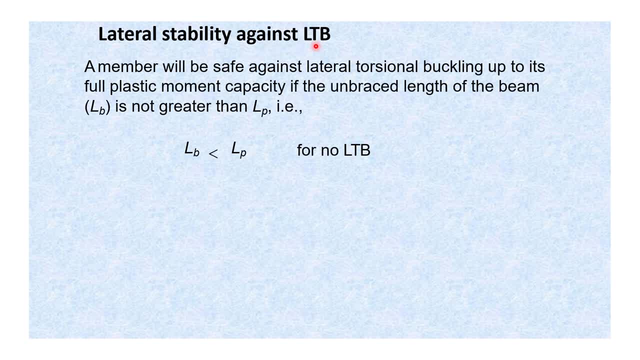 lateral stability against lateral torsional buckling. so first criteria: a member will be safe against lateral torsional buckling means there is no chance of lateral torsional buckling. but there is a length criteria. if the length limit is less than from certain limit up to its full plastic capacity means the the member after yielding will go for full plastic. 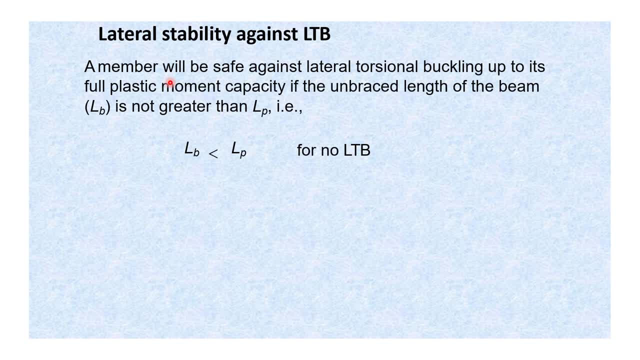 condition, just like i have seen in the stress profiles. if the but the condition is that if the unbraced length of the beam is not greater than lp, if your unbraced length between sports is less than or between any bracing criteria, lb, unsported length is less than lp, then there will 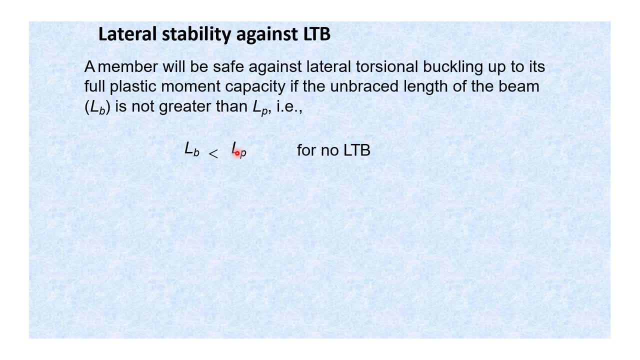 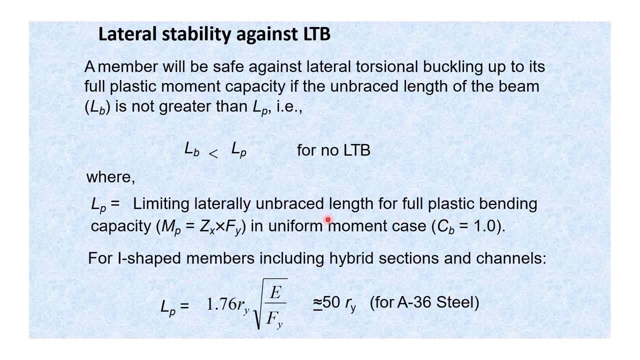 be no chance of lateral torsional buckling. so what is lp? there's a limiting criteria, limiting criteria, literally unbraced length for full plastic bending capacity, ZX into FY in uniform movement case. CB is a modification factor I will discuss again that will be used one for no LTB, no lateral torsion. 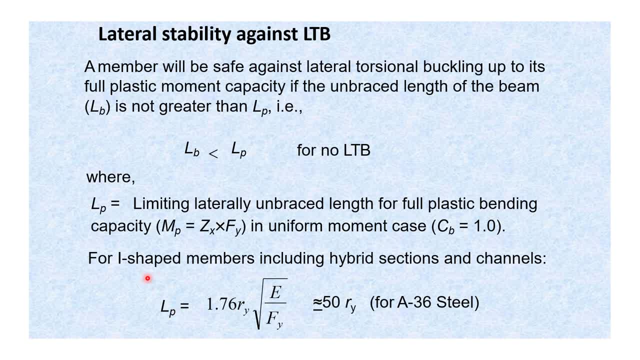 buckling and how LP will be calculated for I shape members, including hybrid sections mean buildup and how troll sections and in China and also for channel section, LP will be calculated equal to one point seven. six are y under root, e over FY, or simply you can approximate for a 30. 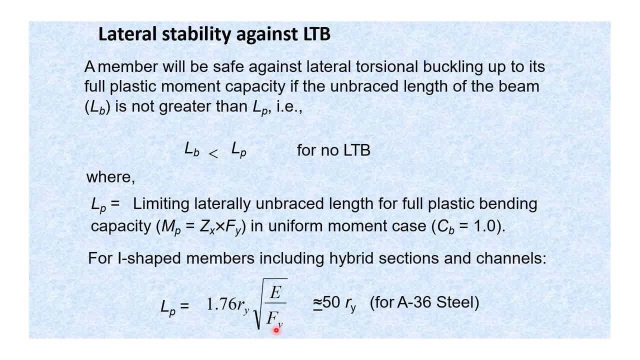 60, 30, 60, when you put FY 250 mega Pascal e 200 giga Pascal, then you will get 50 are y okay? radio of gyration and if you want to calculate for a 30, 60 gyration, for a 30, 60 gyration, for a 30, 60 gyration, 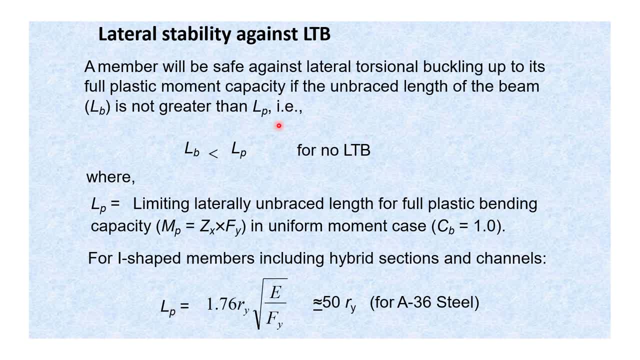 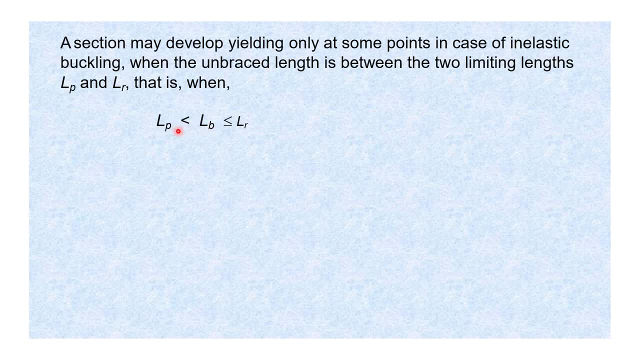 second criteria: if our length is less than L, greater than LP- now our length in length is LP but less than LR- a section may develop shielding. shielding will start only at some points. in case of inelastic buckling. when the unbraced length is between two limits, LP and LR, yielding will start.